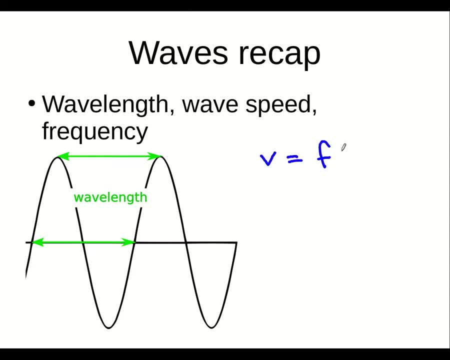 velocity is equal to the frequency times, the wavelength, and also that the time taken for one wave is t, which is equal to one over the frequency. So that's all about the wave velocity, and I want you to see in this video what the wave velocity and wave length are related to. It's this equation that's the most relevant today. 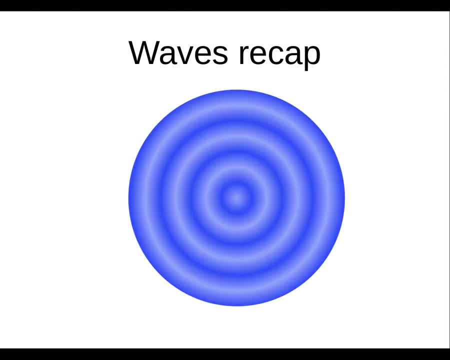 So the wave speed, the wave frequency and wavelength are all linked to each other. If one changes, then at least one of the others has to change. If we look at waves from the top down, these might be ripples in water. then they spread out in these directions. 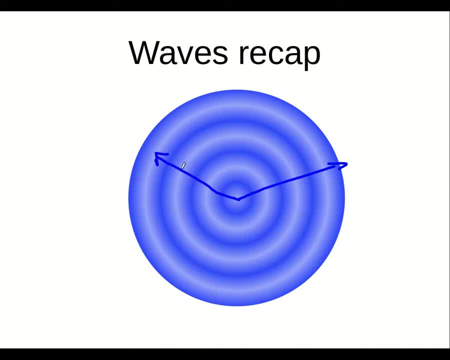 draw the direction of waves. what we're actually doing is drawing a line at 90 degrees to the wave fronts, and the wave fronts are the peaks or troughs of the wave. okay, so these white lines correspond to the peaks and the dark blue lines corresponds to the troughs of the wave. and as the wave moves outwards, 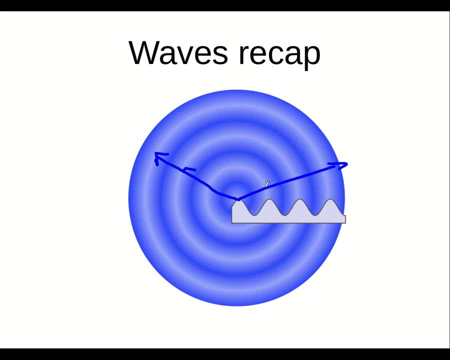 or just moves, then the direction of that is determined by the arrow which is at 90 degrees to these lines here which we call the wave fronts. the distance from here to here and the distance from there to there is the same and that's the wavelength of the wave which you can see from this here. so that is one wave. 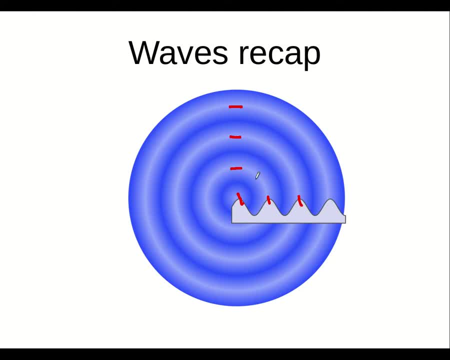 length, that's another wavelength. if I was to stand here and count the number waves go past every second. that would give me the frequency and that would be linked to how fast the wave was traveling in that direction and the wavelength okay. again linked to this equation v. 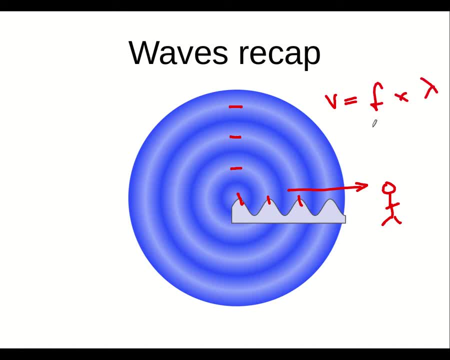 equals f times lambda, so the frequency would be equal to the wave speed over the wavelength and that would be the same everywhere. so if i was over this side observing the same waves, then because they're traveling at the same speed and have the same wavelength, they would appear to have the same frequency. 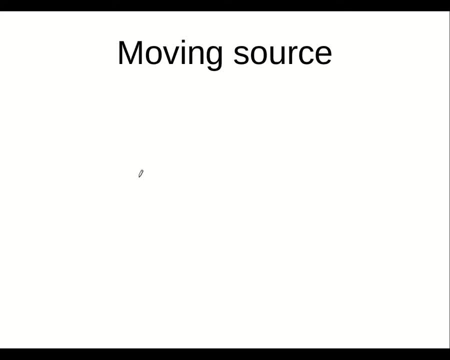 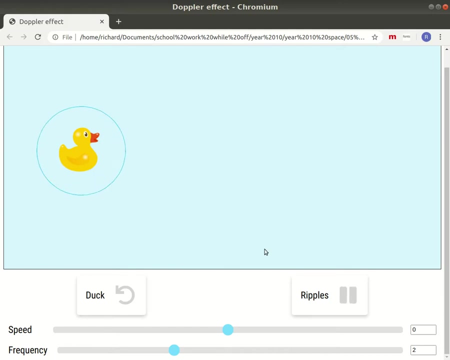 things get a little bit different if the source of the wave is moving. so instead of dropping a stone into the water and creating ripples that spread out, if there was something that was moving, creating the ripples- for example, a duck bobbing up and down on the surface of the water- here we've got a little simulation um of a duck on water. 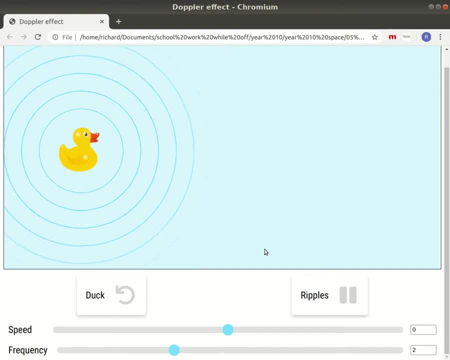 and the ducks bobbing up and down, creating ripples which are spreading out in all directions at the same velocity. and again, if i was to stand here, then i'd observe those waves at the same frequency as if i was to stand here, because the wave speed and the wavelength 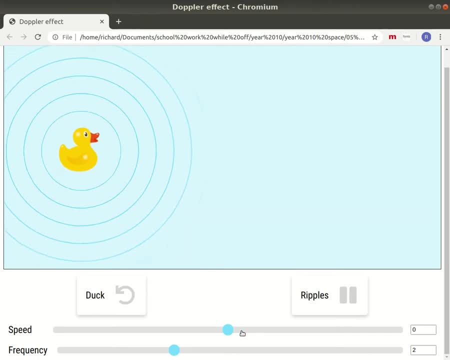 are the same. if, however, the duck is moving, you'll see the waves in front become closer together and the waves behind become further apart, so the wavelength is effectively decreased, and that's because the duck moves forward in the time it takes before the next wave is made. 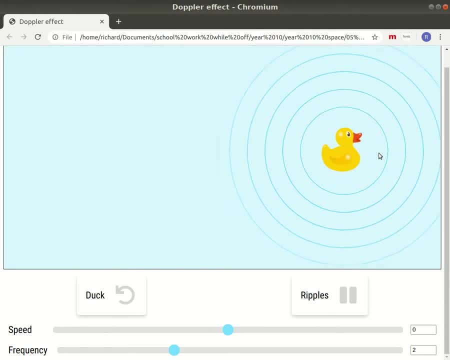 so it catches up with the previous wave a little bit and the faster the duck goes relative to the speed of the wave, the closer those waves get together. so if the duck were to go really fast, you can see the wavelength now in front of the duck or in front of the direction he's traveling is very, very small and the wavelength behind the duck 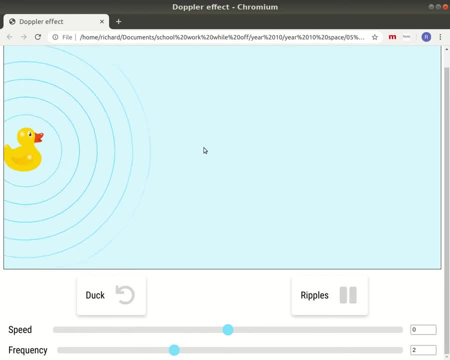 has increased significantly. now the waves are traveling at the same speed in all directions, but the wavelength has changed. so where the wavelength has reduced, according to our equation, the frequency must have increased and, conversely, where the wavelength decreases, the frequency must have decreased, because the wave speed is the same. 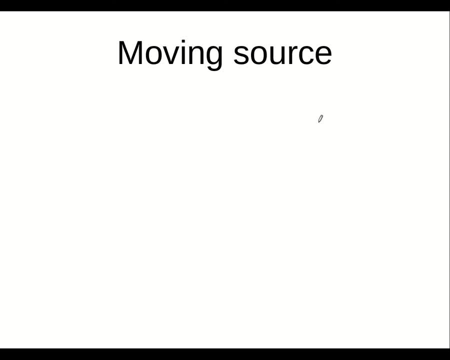 so the doppler effect is the apparent shift in frequency of a wave due to either the source or the thing that's observing the wave moving. it doesn't matter if it's the thing that's producing the wave moving or the thing that's observing it moving towards or away from it, as long as they're.